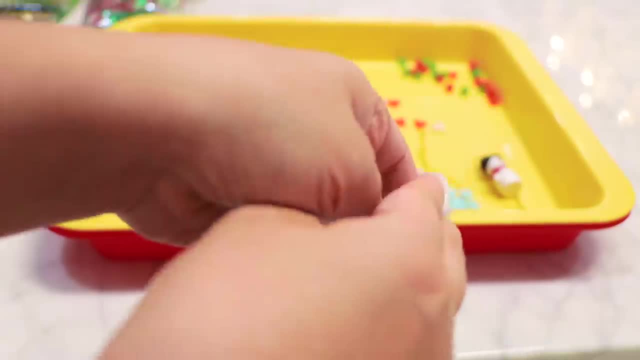 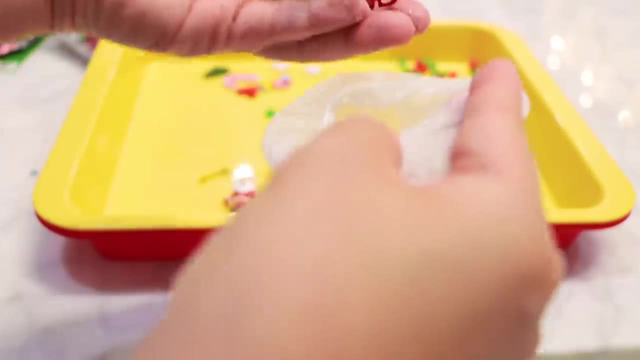 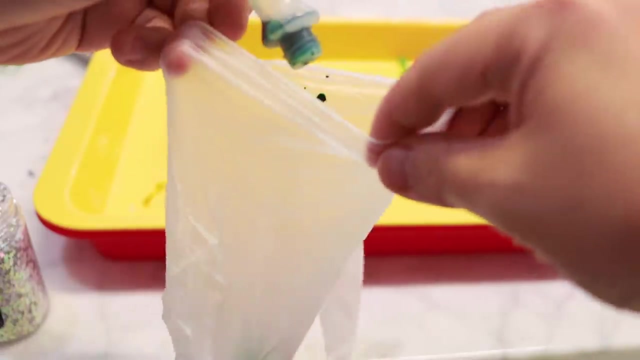 Here I'm going to put in a Christmas tree some other fun things, Stocking Little cute reindeer, Some fun Christmas patterns. Put it all in here, Some glitter. Then add in a few drops of food coloring- I'm going to use green. Drop it in there. 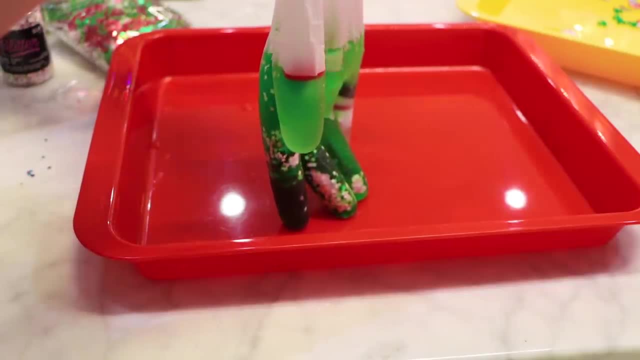 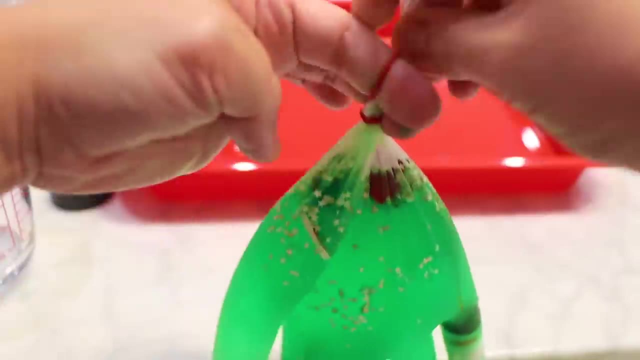 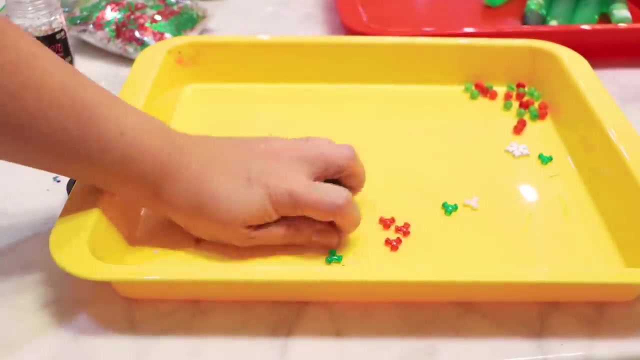 Then fill the glove up with some water. Fill it up three-fourths of the way And, once you're done, tie it with a rubber band. Whee, And here's my first hand For my second glove. I'm going to grab all this real cute. 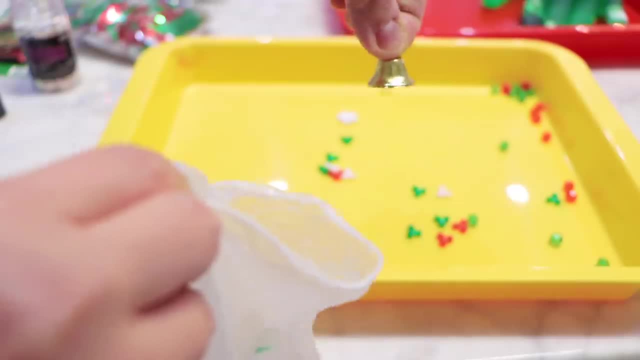 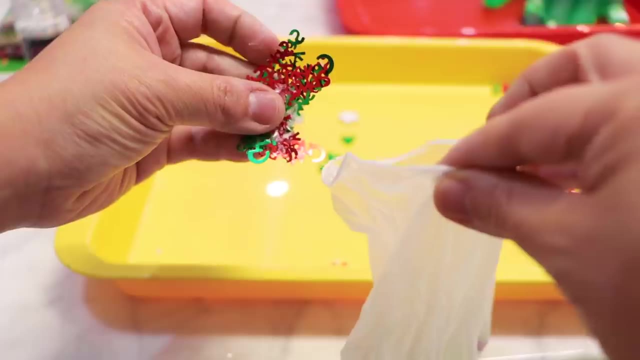 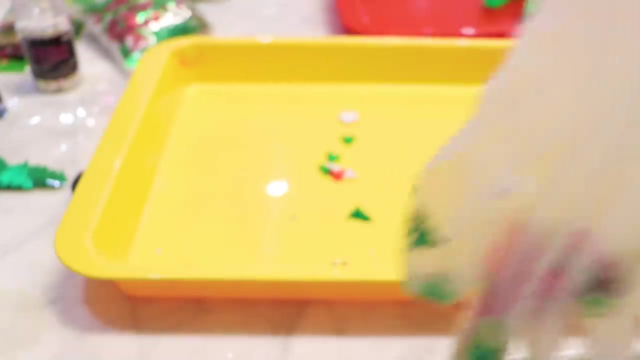 Hi Santa Claus, He goes into the glove. Cute little Bill Into the glove. Some fun Christmas trees, Some Christmas words And some fun glitter. Who doesn't like glitter? Then a few drops of red food coloring. Then add water. 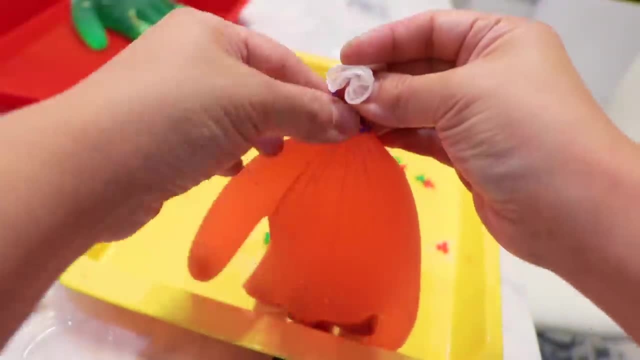 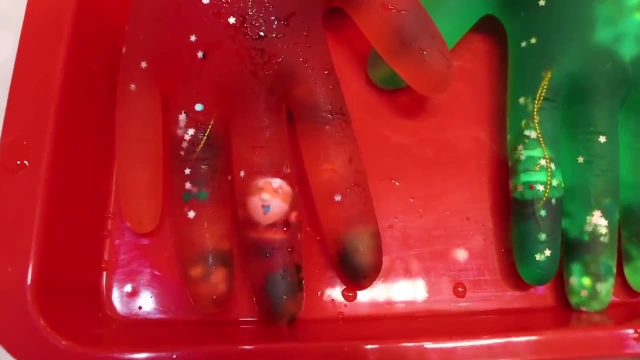 Once you're three-fourths done, tie it with a rubber band. Okay, there's my red one. Look, I see Santa Claus, Do you guys see it? Once you're done, just put it in the freezer. There it is, I put it in the freezer. I'm going to keep it overnight. 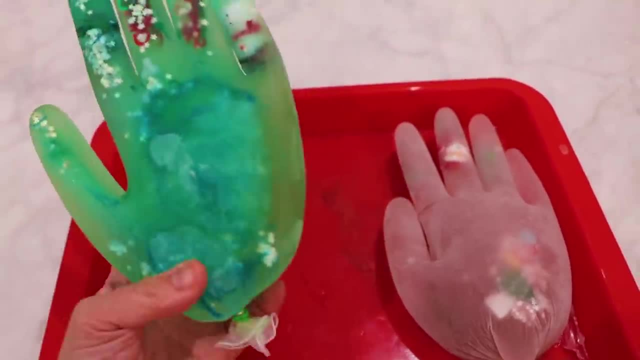 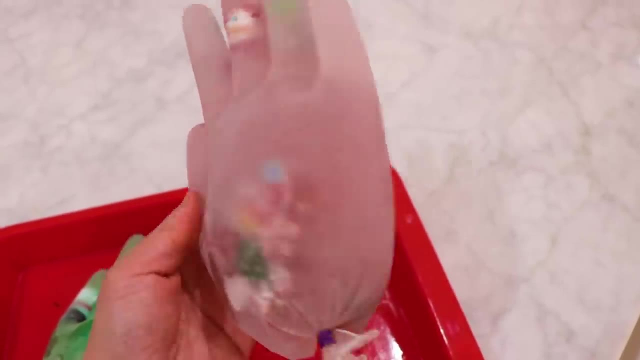 Once it comes out here, it's all frozen. Do you guys see it? It's rock solid Hard. The red didn't stay very well. Should have added more red food coloring, but it comes out pretty good. Do you guys see Santa right there? 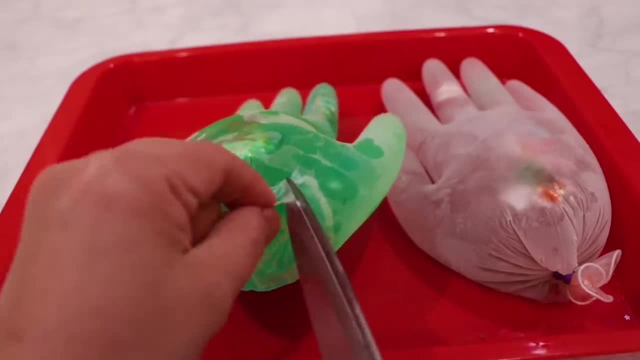 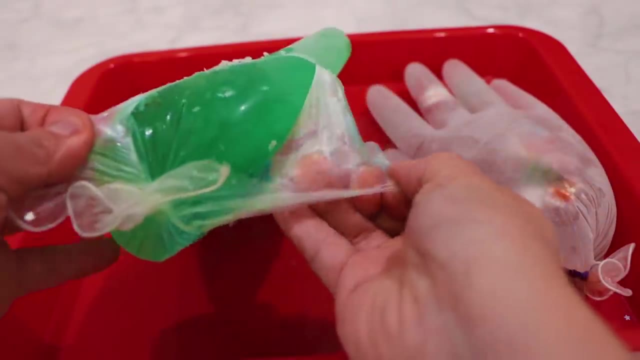 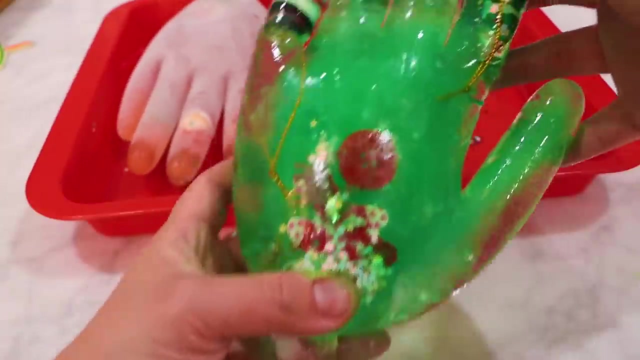 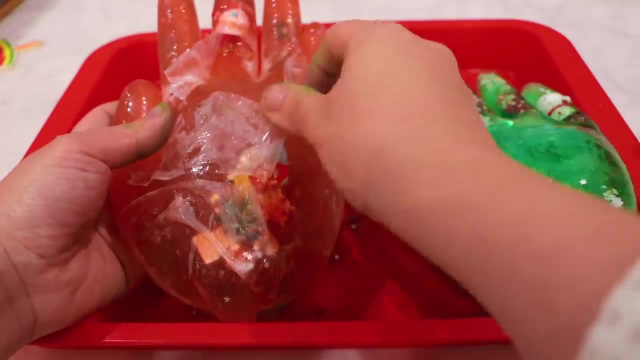 Next, open up the rubber band and then cut And Pew. Be very careful of the fingers and thumb. Once you're done, you'll have something like this: Isn't that cool? Look, be a snowman. Okay, here's the other one. 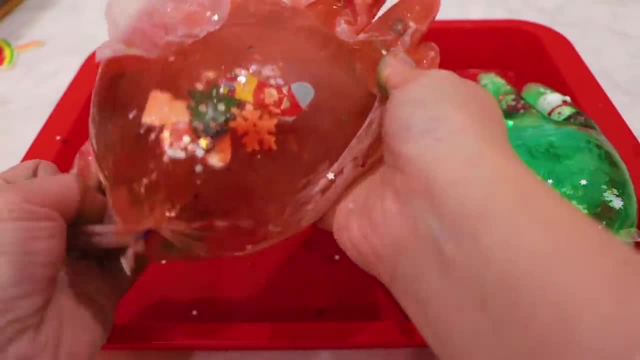 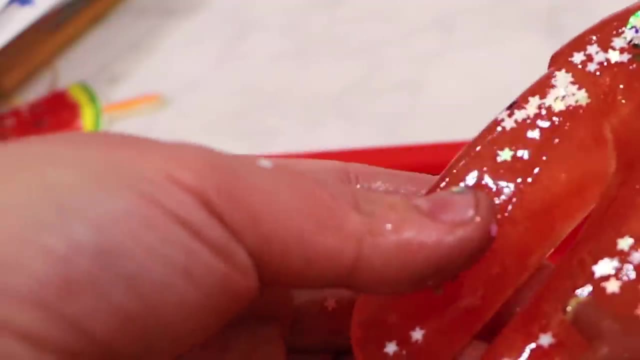 Just pew and cut away. Look there's Santa. Okay, and it looks like this. But guys look, I broke off the thumb. Oh, no, So okay, it's so fun. Look there's Santa. Okay, let's get started. 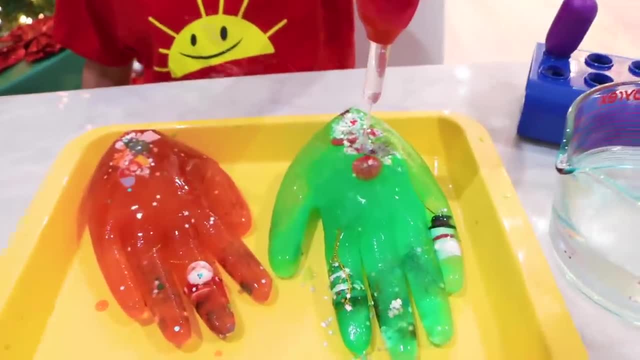 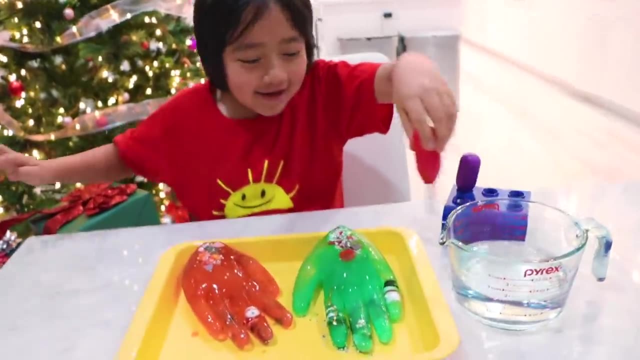 I'm going to try to melt it with some warm water. Hmm, It's working a little bit. Wait. wait, I can feel the objects. It's working. Okay, Did I get the button out? I got the button out. 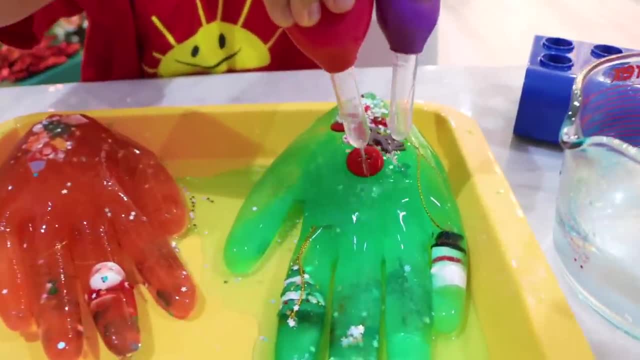 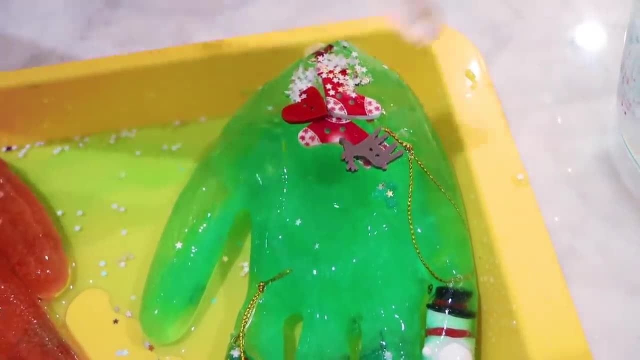 There you go And there, I think this time I'll be able to free something. Oh, wait, wait, wait, I freed it. I freed socks And a heart, Heart And socks. Okay, Okay, Okay Okay. 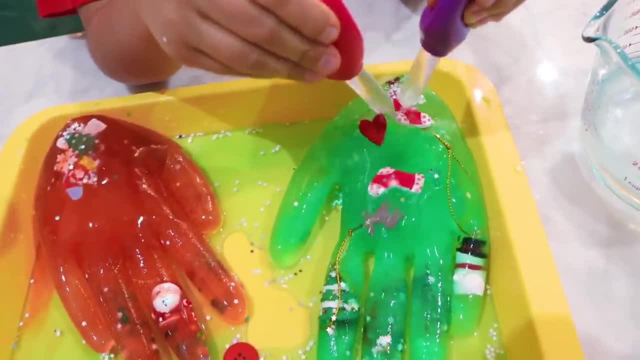 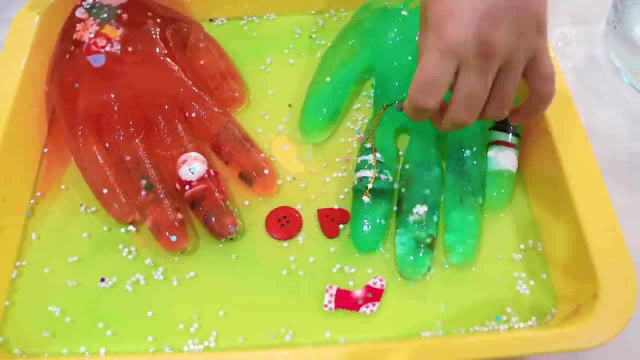 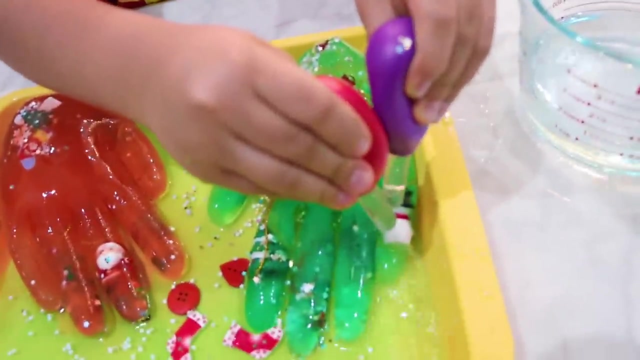 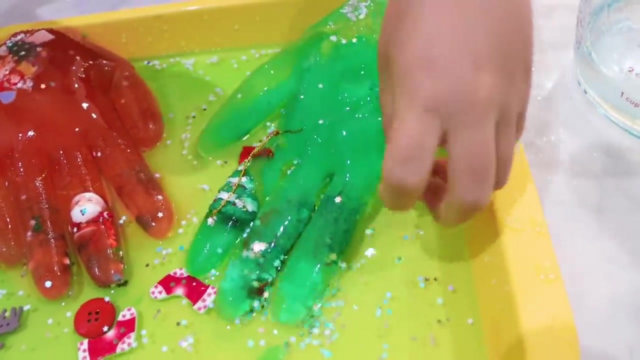 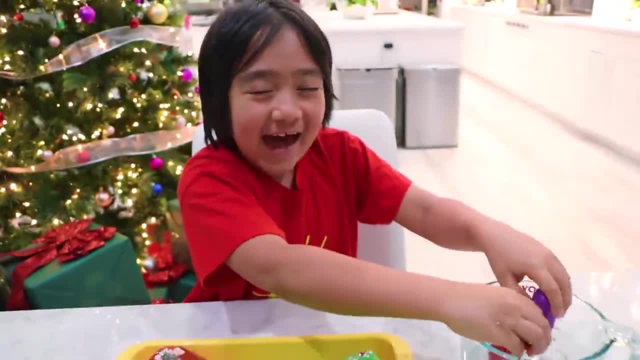 Okay, Okay, Oh, there's another sock. I don't know what I should do. Let me do something else. I got socks And a deer. Oh, and another sock. Don't worry, snowman, I'm coming for you. 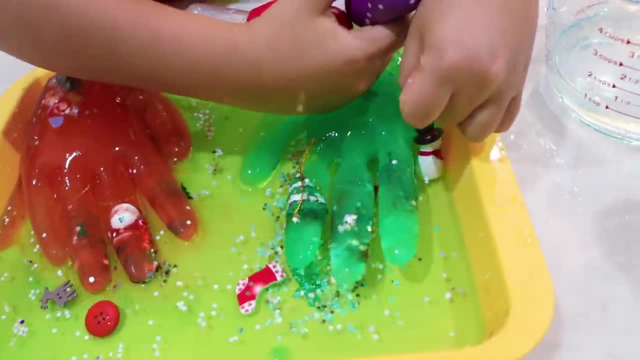 I think I have to put all the water in one spot. I think the snowman's out. Oh oh no, There's a chain. Yeah, got him out. yes, Okay, guys, I'm gonna try to pick it up. 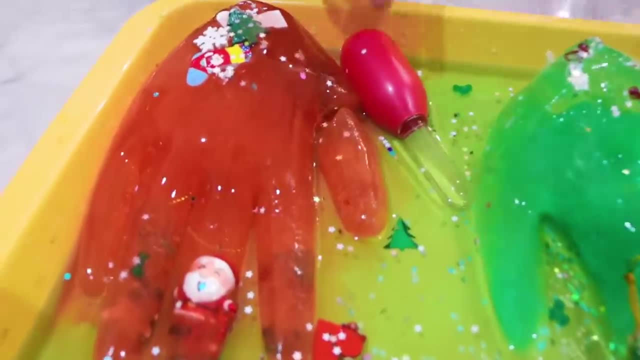 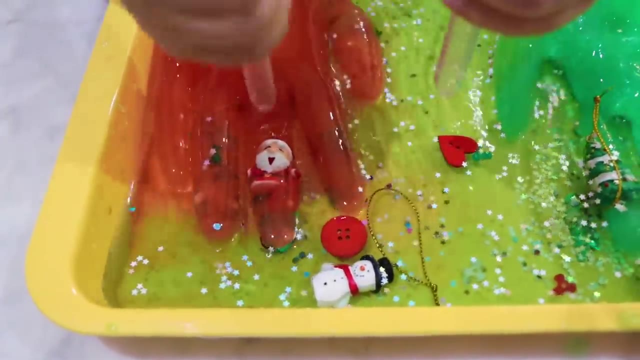 Oh, it's super cold and it's missing a pinky. ah, This one's also missing a thumb. Okay, Santa, I'm gonna try to rescue you now. I put all of the force right here. Oh, there's another golden chain. no, 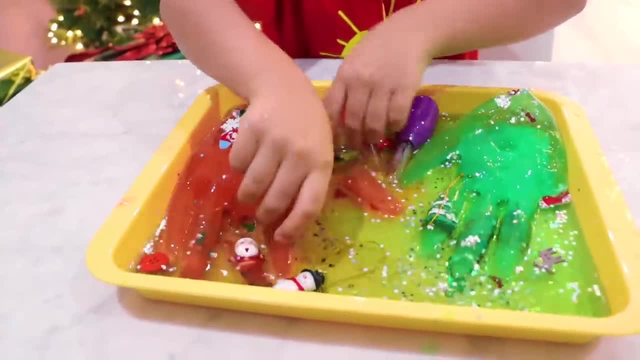 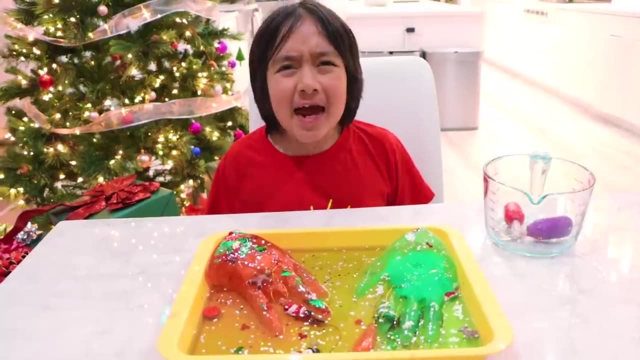 Where does the golden chain lead to, Guys? the chain is super long. It's all the way up to here. Ah, what do I do now? I have an idea. I'm gonna go get a mallet, guys. Okay, guys, I got two of them. 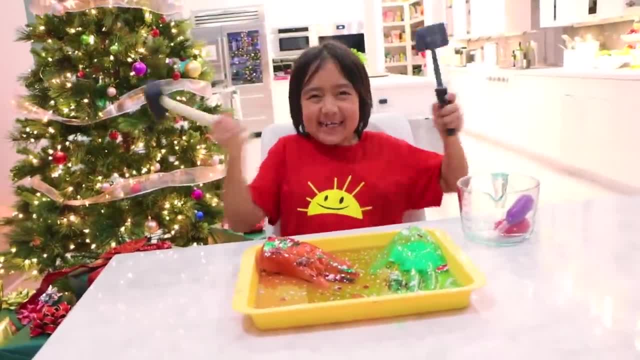 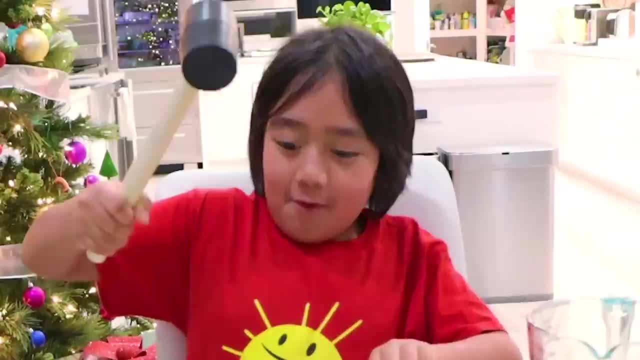 But remember to ask your parents for permission, because my mom said, yes, Right, mommy, That's right. yep, Okay, let's try this one first. I think that one will be stronger though. Whoa, whoa, it's working, it's working. 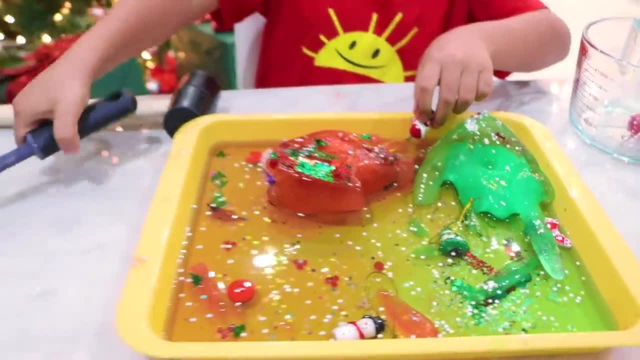 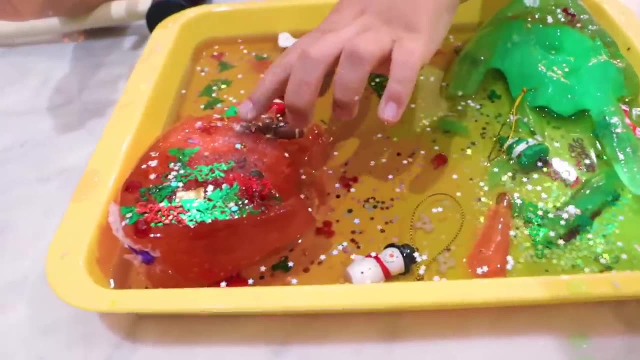 Wait Santa's out a little bit. Okay, maybe I should use this one now. Whoa splash of a lot of water. What's breaking the ice? The ice is shattering. Okay, guys, I'm gonna put some more warm water. 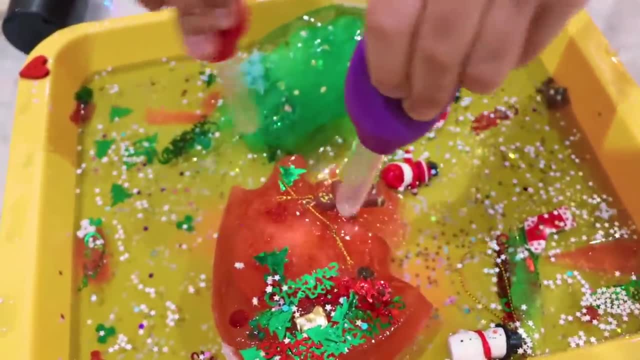 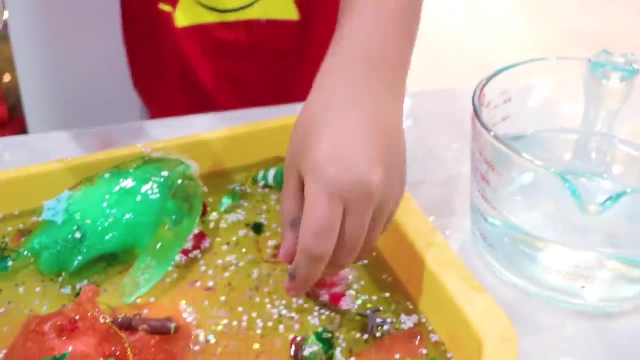 And this time it's even hotter. Whee, I got the chain out, Chain out. I didn't get Santa, I got Santa, Wait, and I got the gingerbread man. Whee, Yes, and the gingerbread man. 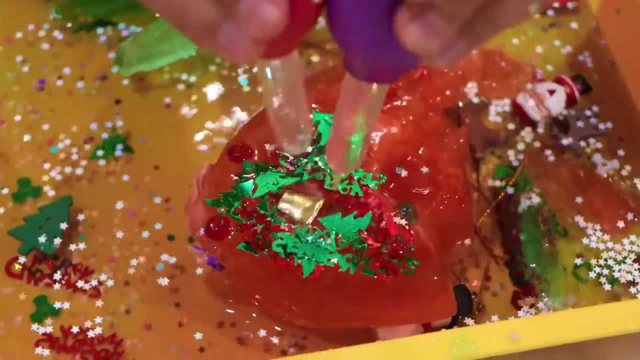 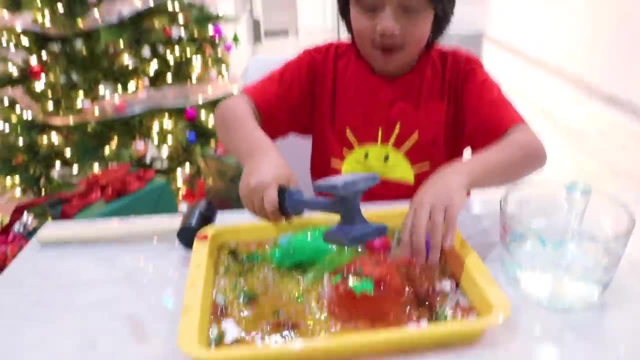 Guys, one more the bell. Okay, Come on, You can get it out. This time I'm gonna use the hammer again. Whoa, whoa, whoa. Wait, did I get it out? Wait, I got other stuff out. 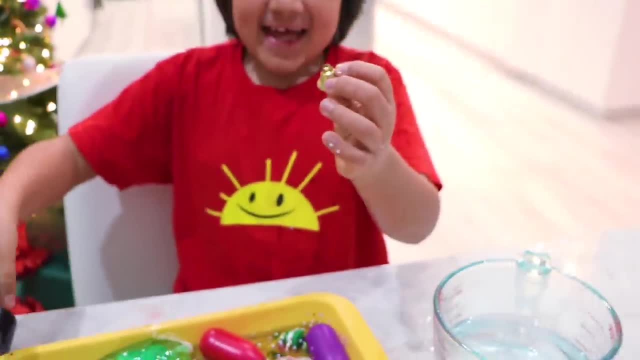 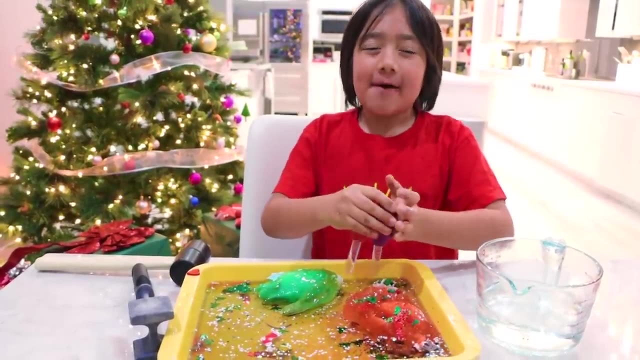 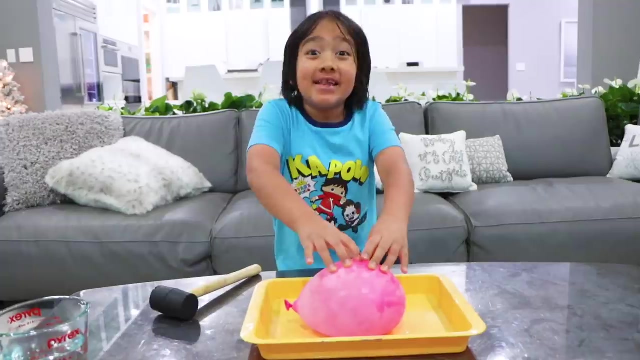 Wait, I got the bell. I got the bell out. Yeah, Okay, guys, I think I got everything important for Christmas out. Hey guys, today I'm doing the Freezie Animal Challenge. Mommy, put a shark inside this balloon. 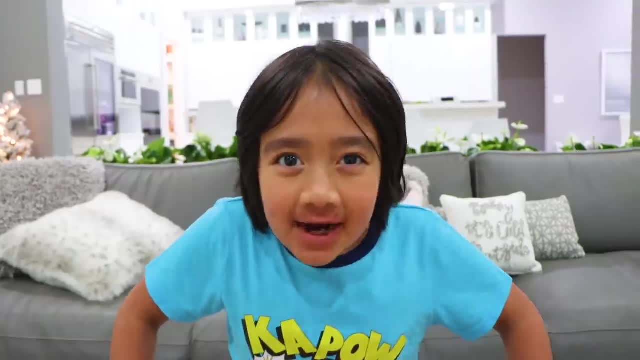 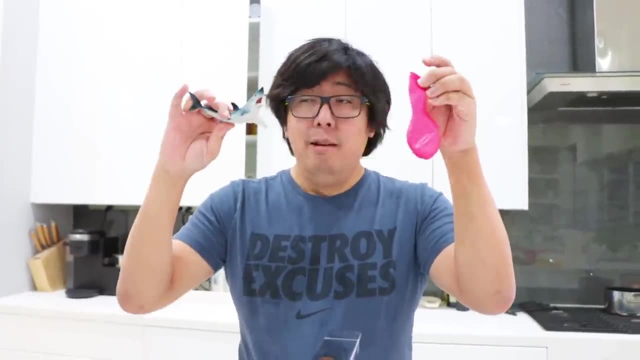 And this balloon is filled with ice And I'm gonna have to free the shark from the balloon. And first, here's how Mommy did it: First grab a balloon, Then get your favorite toy. Carefully put the toy inside the balloon. 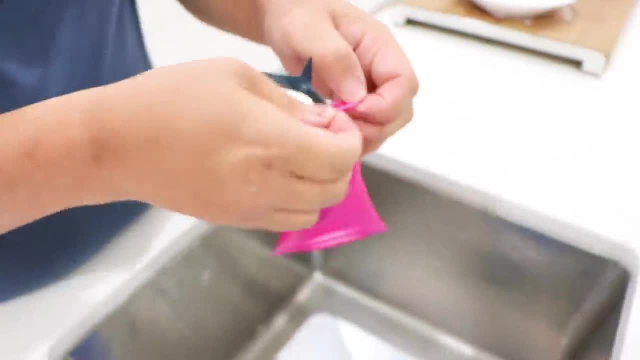 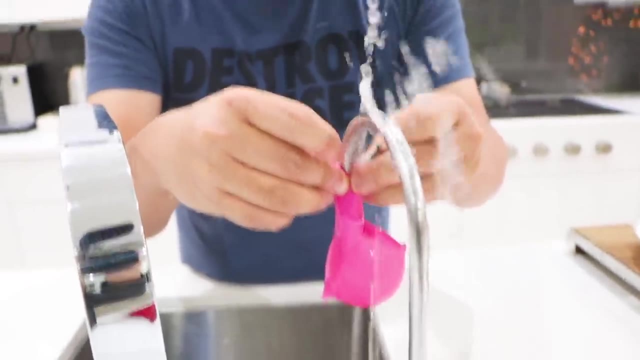 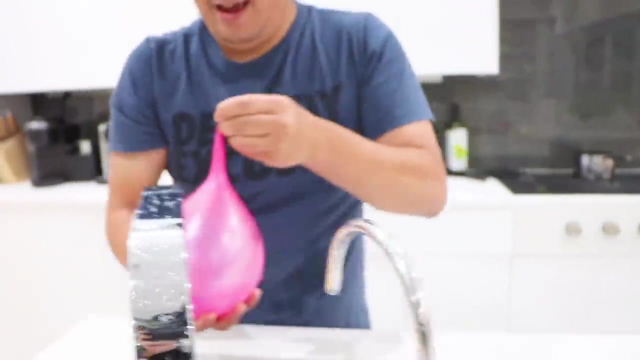 Did I mention carefully, Once the toy is inside, fill the balloon with water. Oopsie Carefully not to splash water everywhere. The balloon will get bigger and bigger. Then remove it and put it on the tray. Next, tie the balloon, so the water. 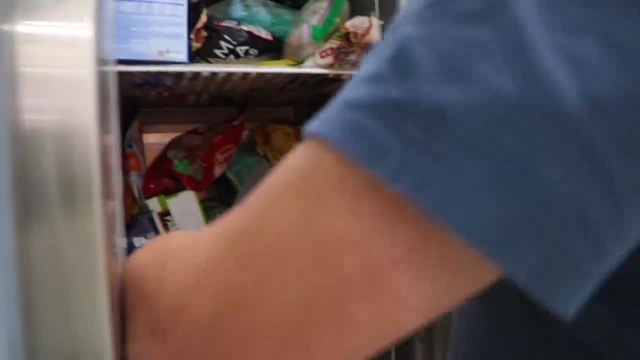 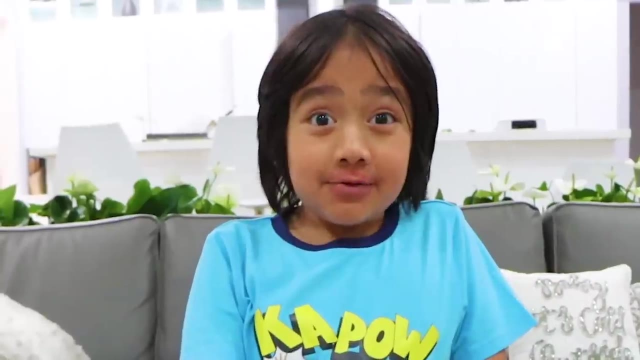 won't spill out everywhere. Next, put the balloon in the freezer until the water inside becomes ice. Okay, first I'm gonna try to get rid of the balloon, And also, don't forget to ask a grownup for help. I have Mommy here. 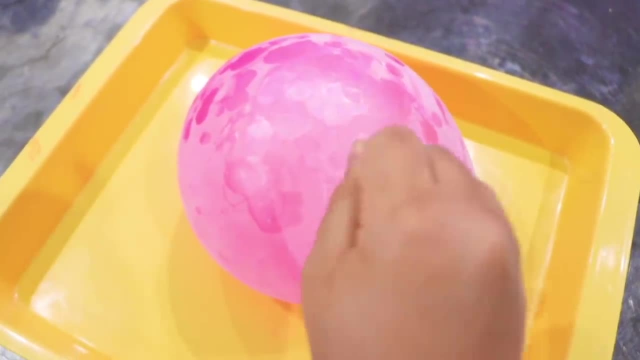 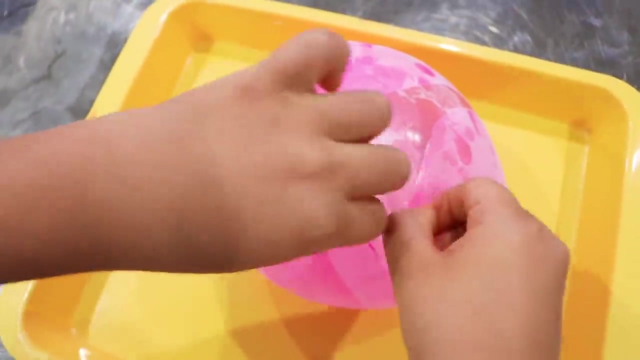 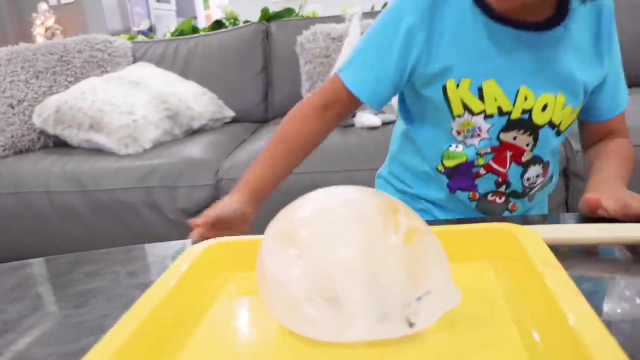 Hi, Won't you work out? It's not breaking. Whoa What It's not breaking. It's super strong, What I'm gonna take the balloon off and you won't even see a difference. Wait, guys, I think I see the shark inside somewhere in the ice. 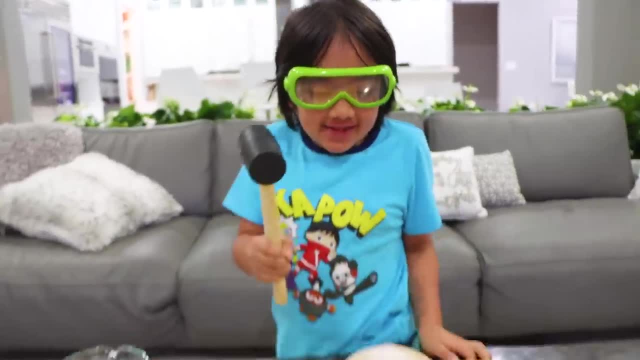 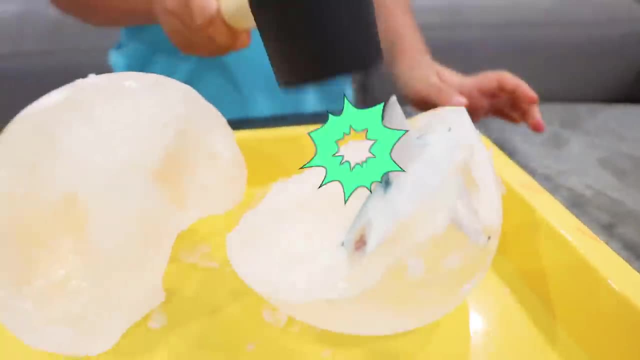 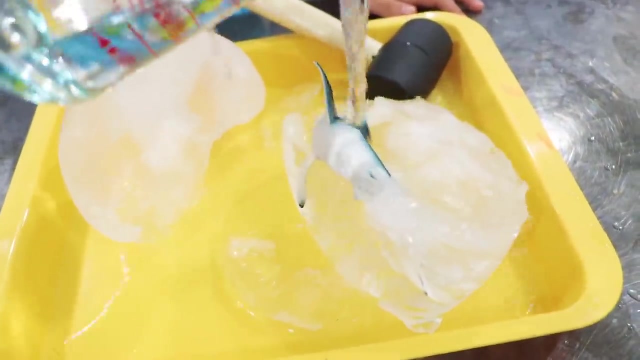 First, I have my goggles, Just in case. Okay, let's get started. We already cracked it. Ah, I see the shark already, but I'm gonna try to use warm water. It's working. It almost got the shark out. 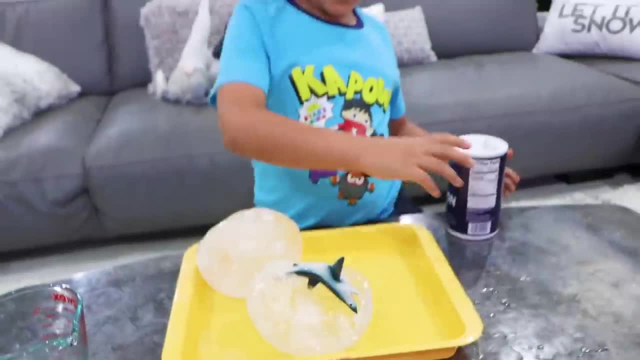 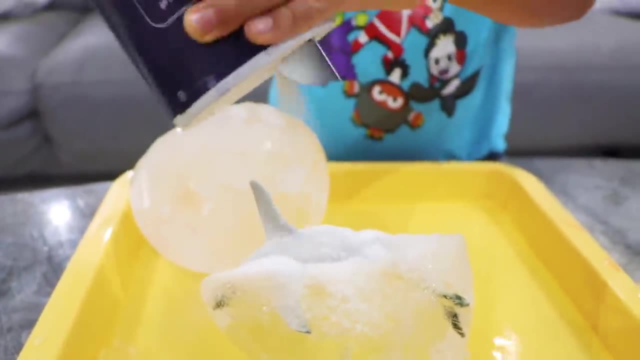 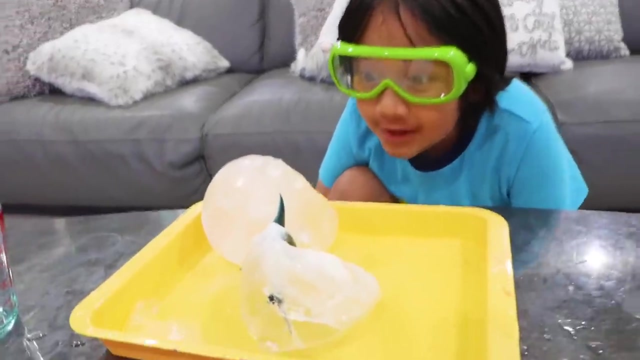 He's right there, but his fin and his tail is stuck. I think that I can use salt. Oh, oh, oh, oh, oh, oh oh, Bam Snow, I hear the ice crackling. guys, It's working. 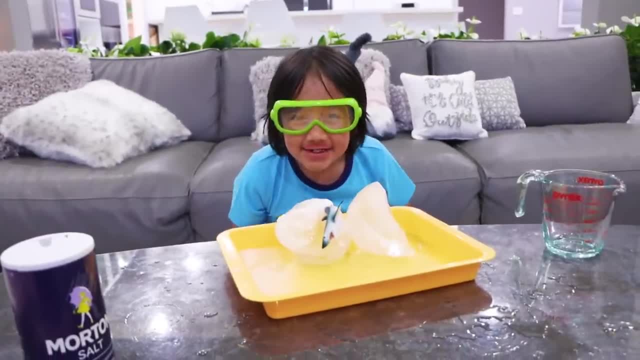 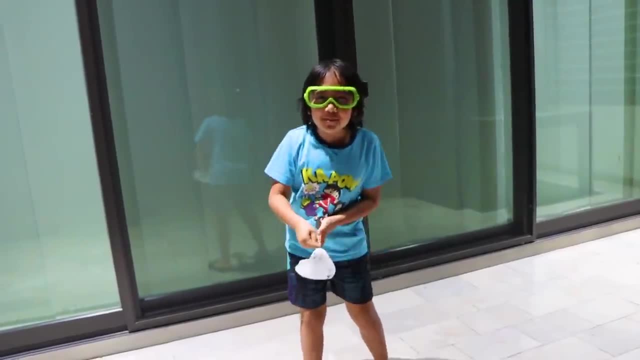 I don't want the shark to crackle. I think I have an idea, Mr Shark, Let's take it outside. Remember I would only do this with adult supervision. Okay, Three, two, one. He almost got out. 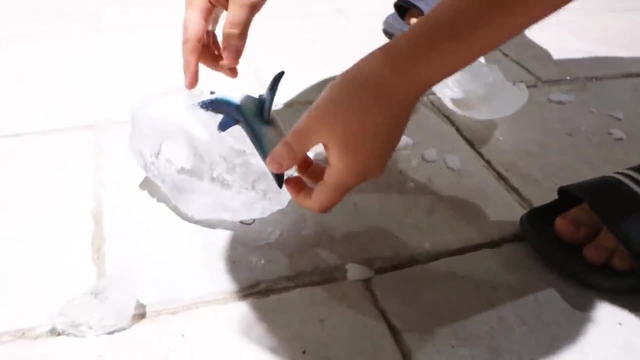 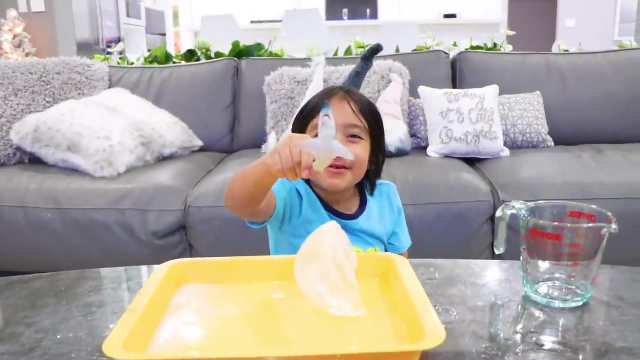 Ooh, can I take him out? No, not yet. His tail is still stuck. Yes, I got the shark out. Thank you for rescuing Mr Shark with me. Bye, Thank you for watching. Remember, always stay happy and rise up. 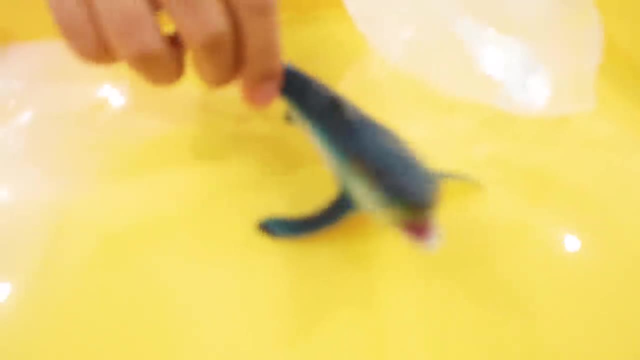 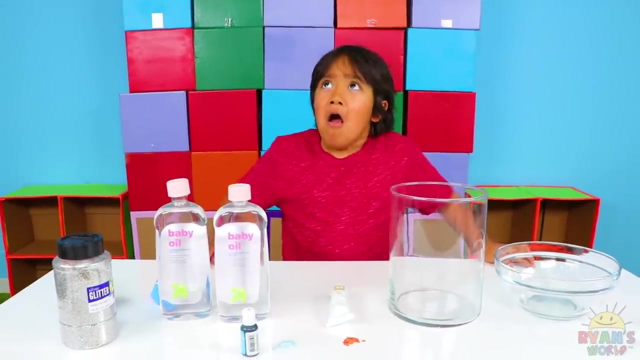 Bye. Shark says bye too. Hoo, hoo, Hoo, hoo, hoo hoo. Hi guys, Today we're making a snowstorm in a jar. I'm talking about snowstorms. I think there's one coming right now. 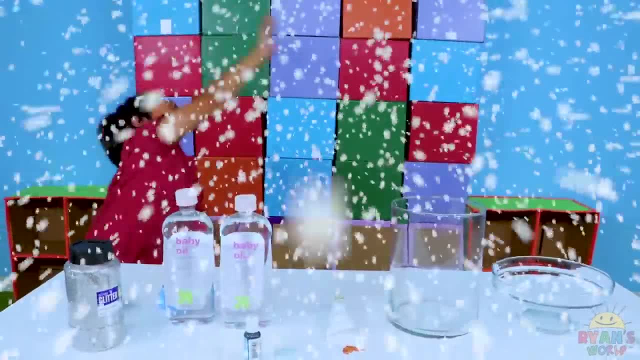 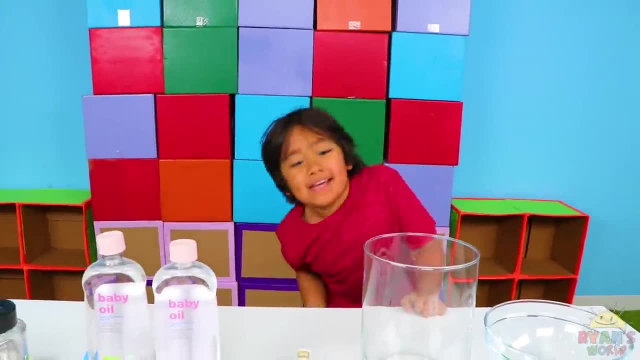 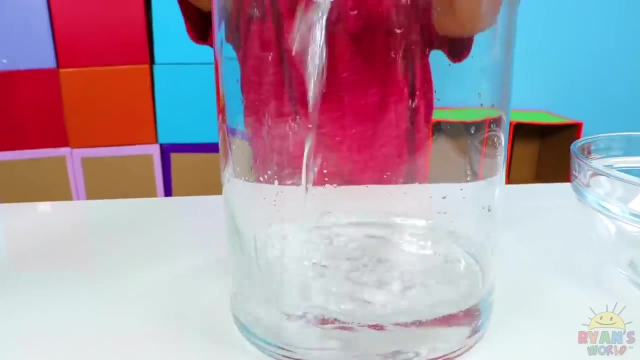 Ah, Ah, Ooh, ooh, Ah, I'm okay. Is it done yet It is Yay. First, you're gonna need baby oil. Oh, okay, Also, we're going to need some. Let's have a look at how much baby oil you actually have in the jar. 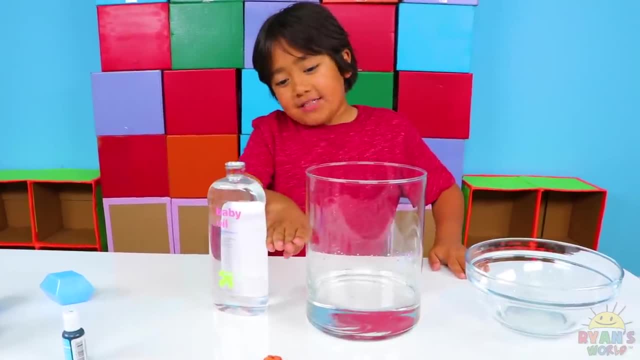 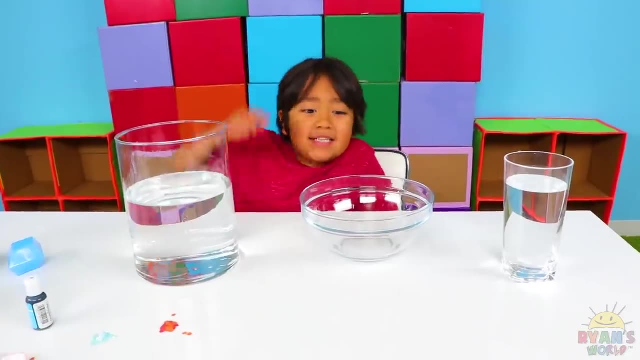 This is the amount of baby oil you can use. This is a huge container, It is, So first we're going to put it in the jar. This is about 1.5 lbs. We're going to fill it. Oh my gosh. 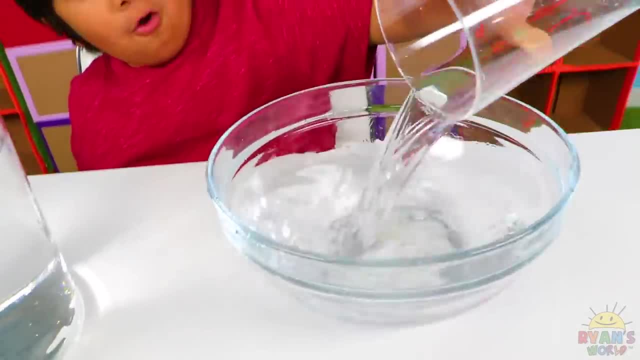 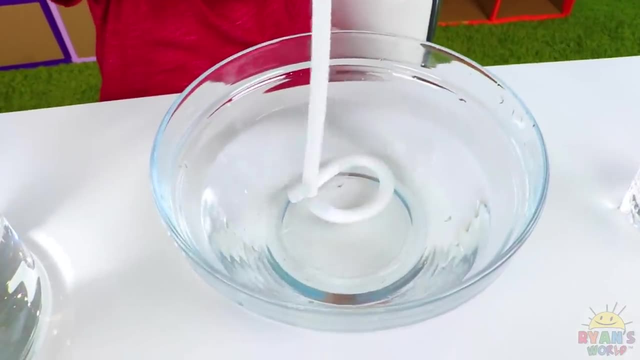 We're going to fill it, And now we need to fill up halfway, so up to here. Next, in your second container, add water, water, water. Next, add some white paint. Alright, guys, let's mix it together. 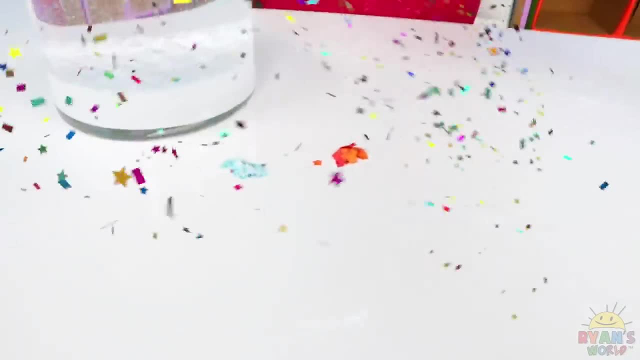 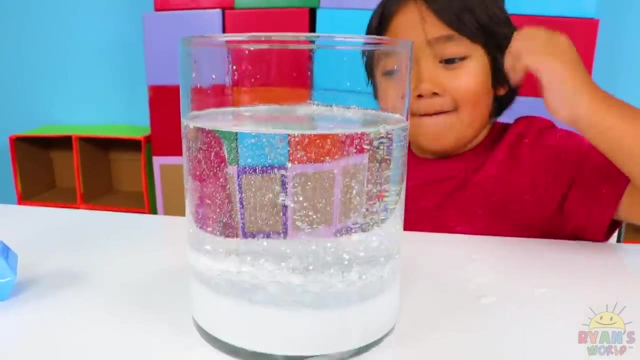 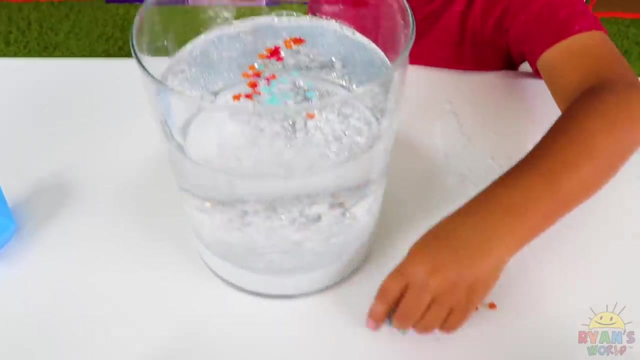 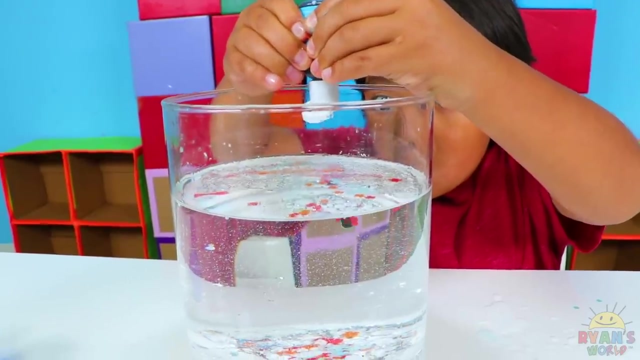 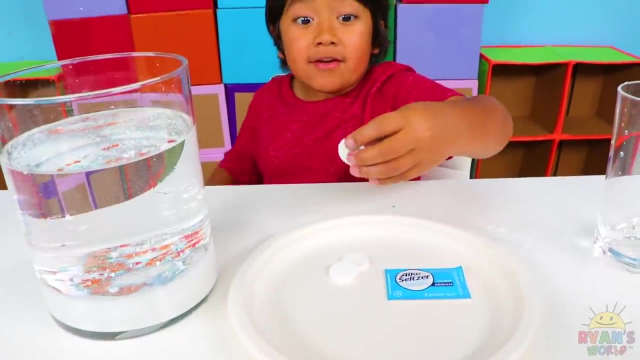 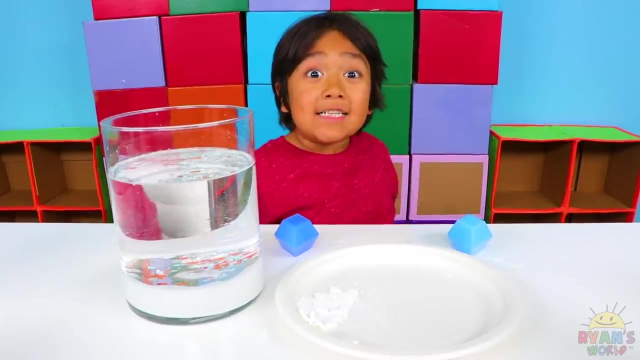 Next, you can add some glitter and some confetti if you want. That's enough. Next, I'm going to add one or two drops of blue coloring. There you go. Next, get some Alka-Seltzer like this and then crush it up. so. 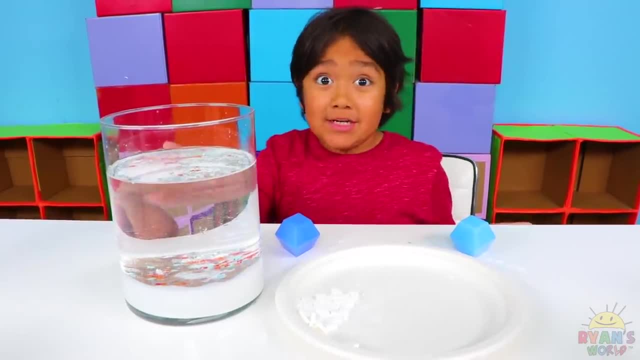 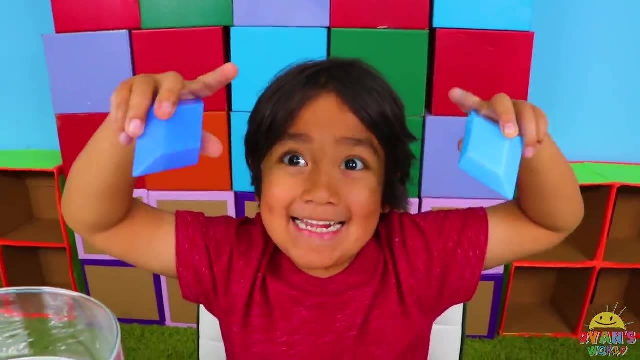 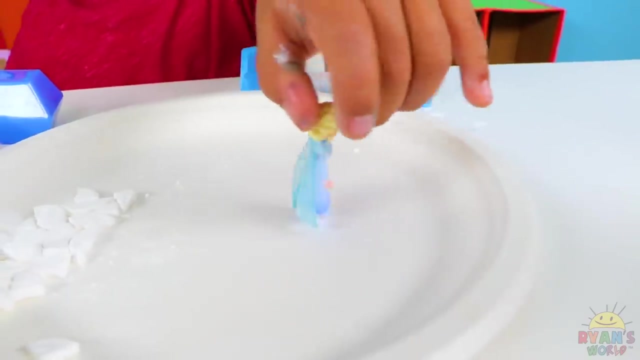 Since Frozen 2 is coming out and it's just like snowstorms, I got me some Frozen blind bag thingies. Let's see who we got. Whoa, we got Elsa. Oh yeah, Alka-Seltzer, This is my Frozen power. 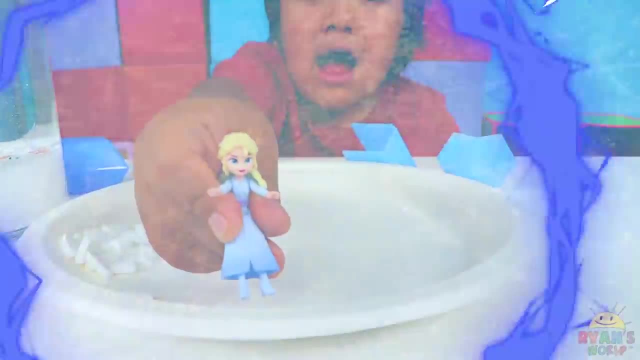 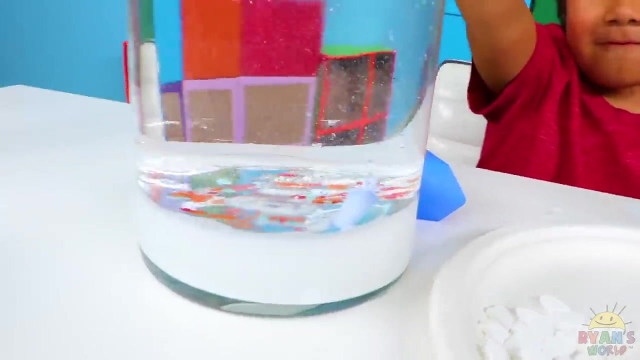 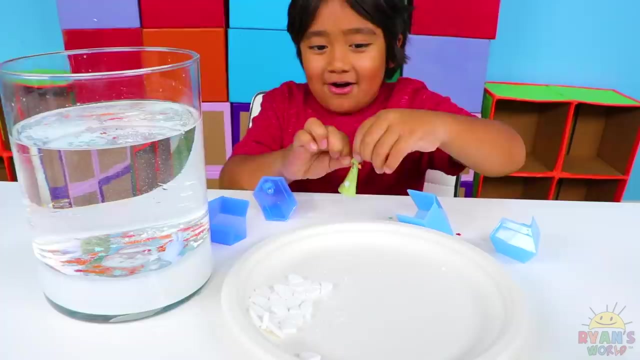 Yah, yah, yah, yah, Ahhhh. No, she's in a snowstorm And we just happened to get Anna. Okay, let's follow Elsa's track. Okay, Do, da, da, da, do, da, da, da, do, da, da da. 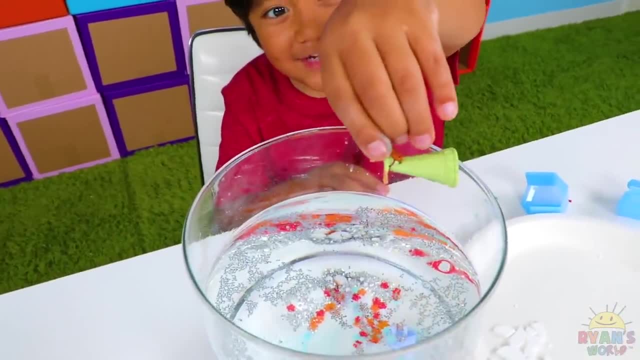 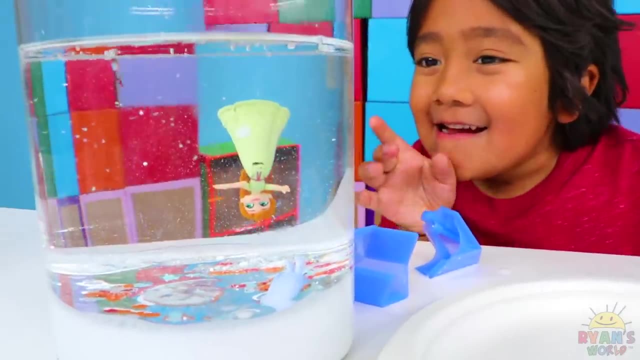 Waah ah, Elsa, I see you down there, I'm going to save you. Waah, waah, waah, Whoa, she's backwards, she's floating, Whoa, Hello, Hi Anna, You have some powers we don't know about. 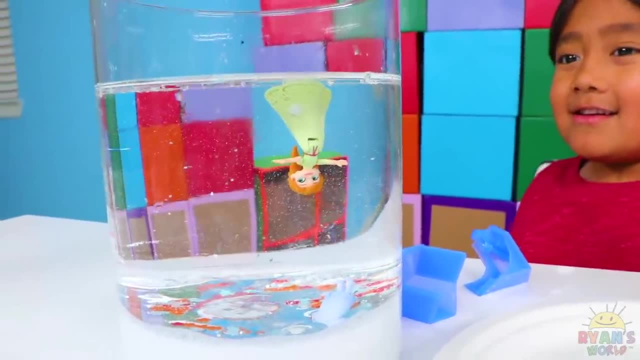 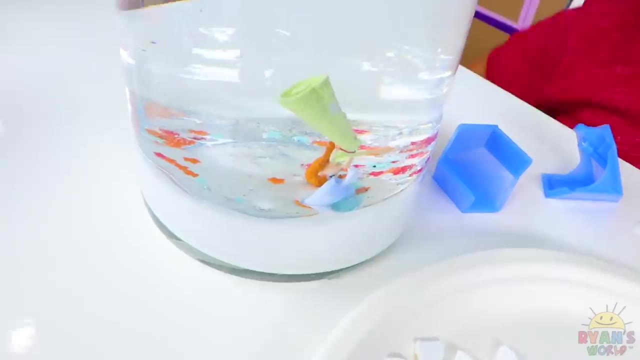 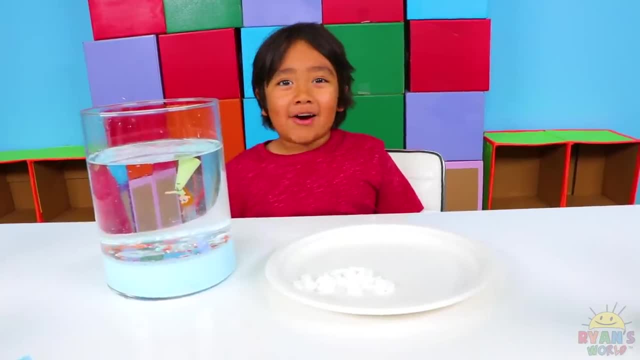 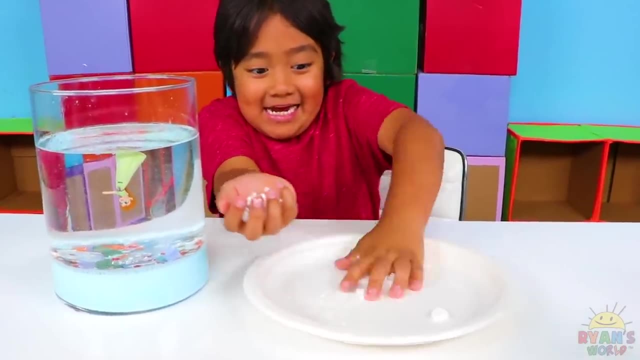 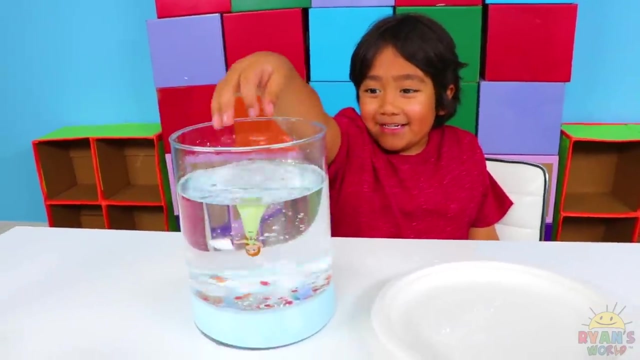 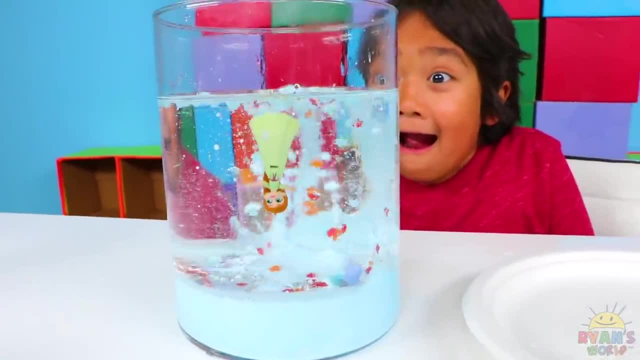 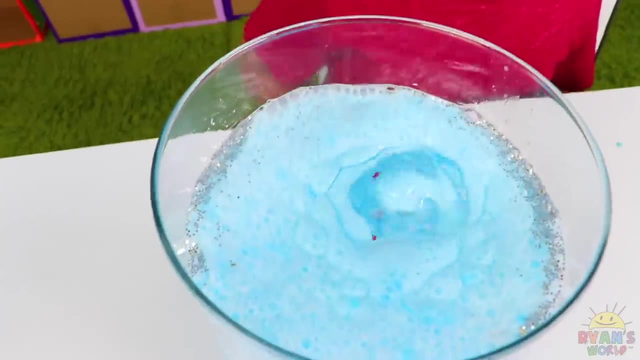 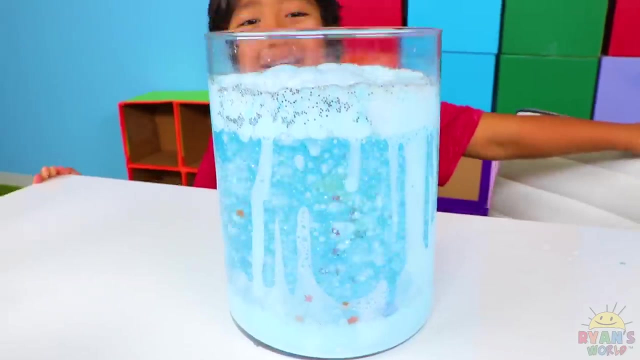 comes. Waah. Everything is going to the top. I'm falling down, Whoa, Whoa, it's popping up. I can barely see anything now. Oh, where's Anna and Elsa? Oh yeah, where are they? Can you guys survive this snowstorm? 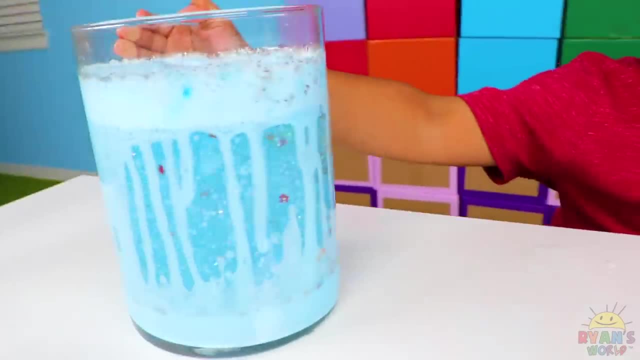 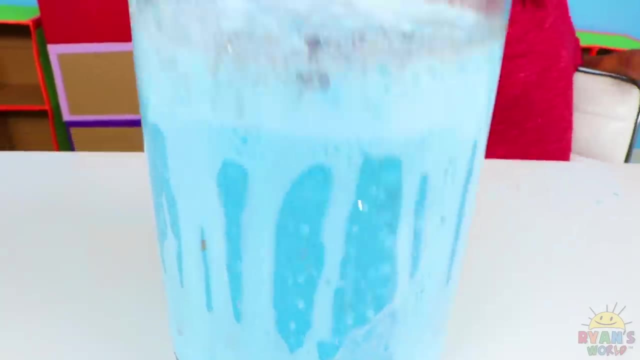 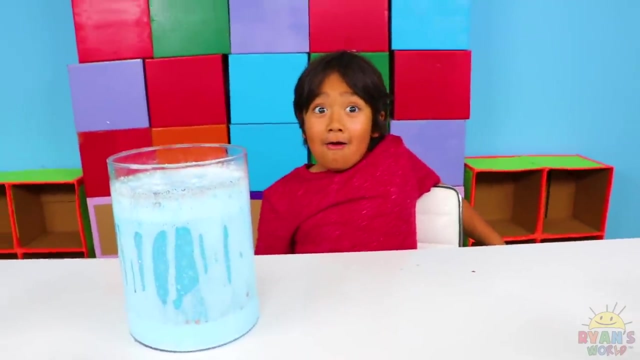 Oh my gosh, Do you see them? No, I see Anna. Oh no, where's Elsa? Anna's right here. I think Elsa's somewhere down there. Oh my gosh, are you okay? They're both drowning. Ryan, watch out, because there's a snowstorm coming too.